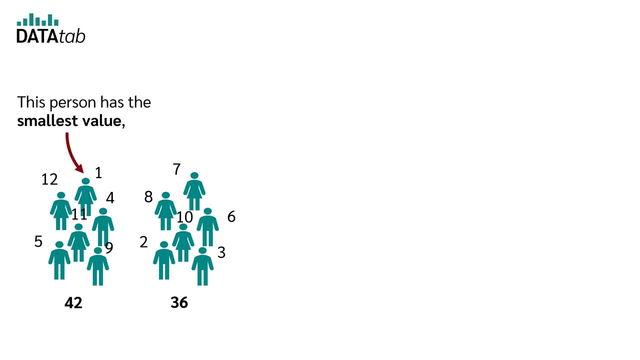 from the smallest to the largest value. This person has the smallest value, so gets rank 1.. This person has the second smallest value, so gets rank 2.. And this person has the third smallest value, and so also gets rank 2.. This person has the third smallest value, and so also gets rank 2.. 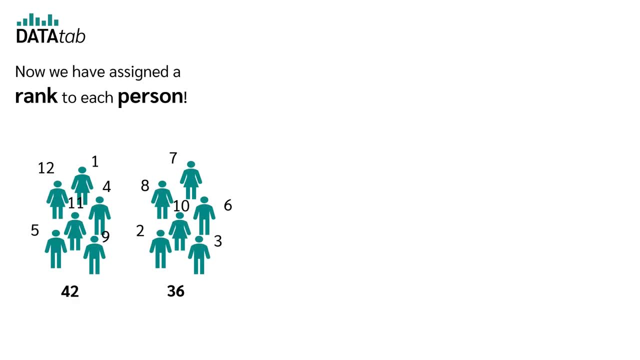 On and so forth. Now we have assigned a rank to each person, Then we can simply add up the ranks of the first group and the second group. In the first group we get a rank of 42, and in the second group a rank of 36.. Now we can investigate whether there is a significant difference between. 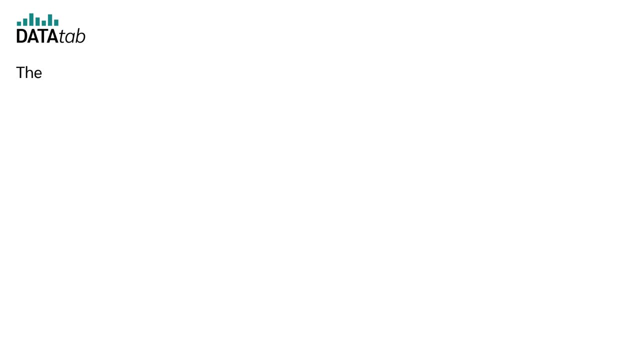 these rank sums, But more on that later. The advantage of taking the rank sums rather than the difference in means is that the data need not to be normally distributed. So, in contrast to the t-test, the data in the Mann-Whitney U-Test do not have to be normally distributed. What are the hypotheses of the? 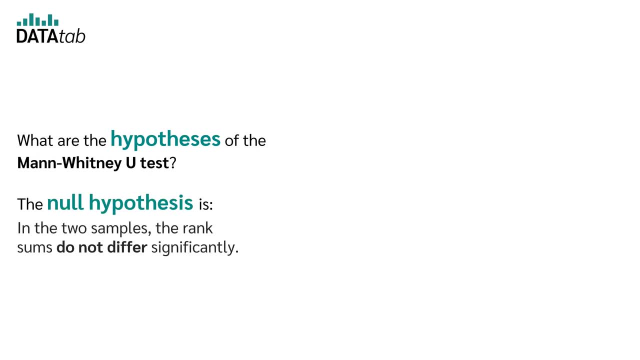 Mann-Whitney U-Test. The null hypothesis is in the two samples. the rank sums do not differ significantly. The alternative hypothesis is in the two samples, the rank sums do differ significantly. Now let's go through the rank sums. 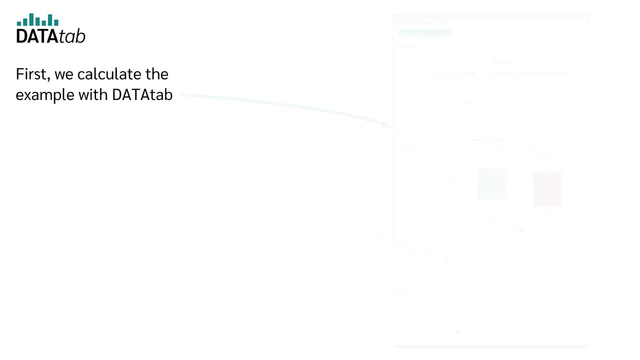 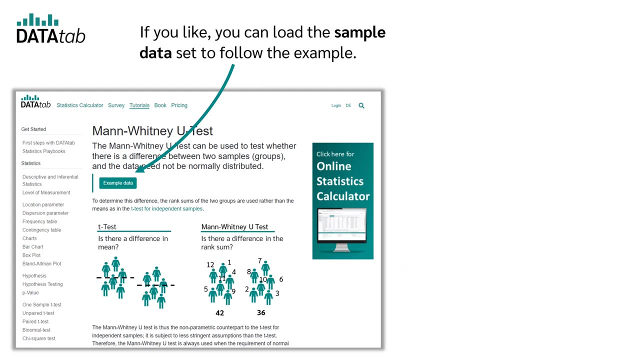 So let's go through everything with an example. First we calculate the example with datatab and then we see if we can get the same results by hand. If you like, you can load the sample data set to follow the example. You can find the link in the video description. We simply 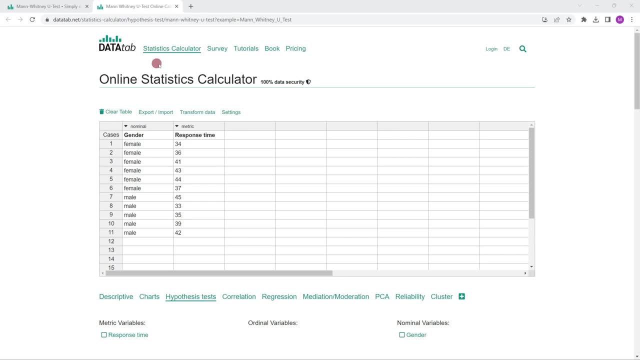 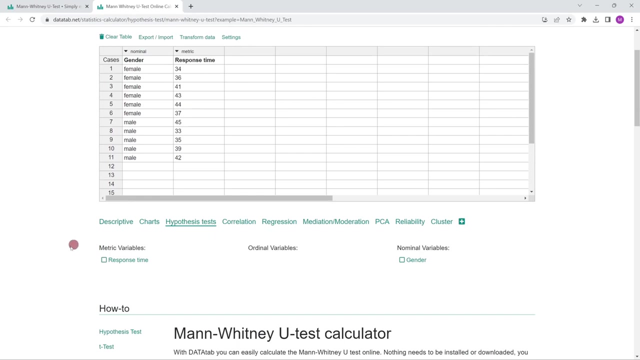 click on datatabnet and open the statistics calculator. I've already loaded the data from the link here. You can also copy your own data into this table. Then all you have to do is click on the hypothesis test tab and then simply select the desired variables. 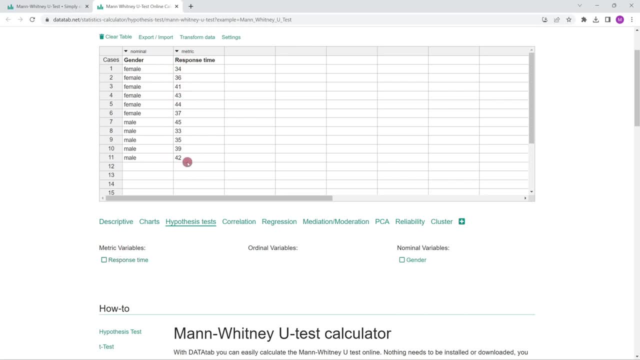 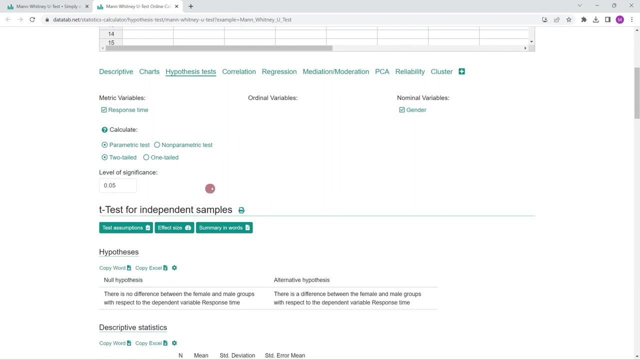 We measure the reaction time of a group of men and women and want to know if there is a difference in reaction time. So we click on response time and gender. We don't want to calculate a t-test for independent samples, but a Mann-Whitney U-Test, So let's just 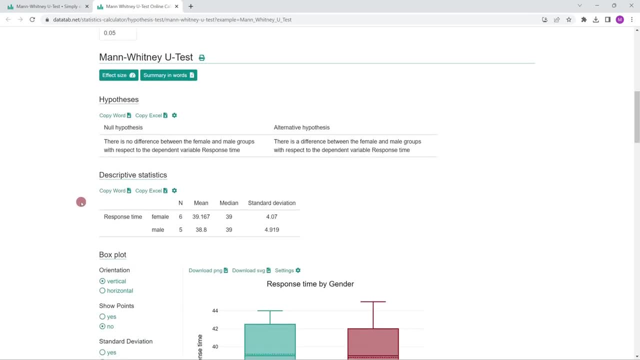 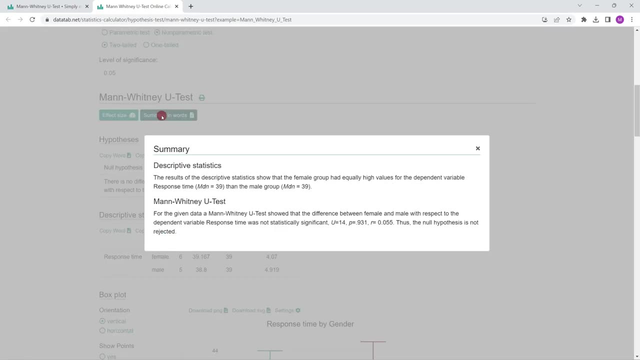 click on non-parametric test. Here we see the results of the Mann-Whitney U-Test. If you are not sure how to interpret the results, just click on summary in words For the given data. a Mann-Whitney U-Test showed that the difference between female 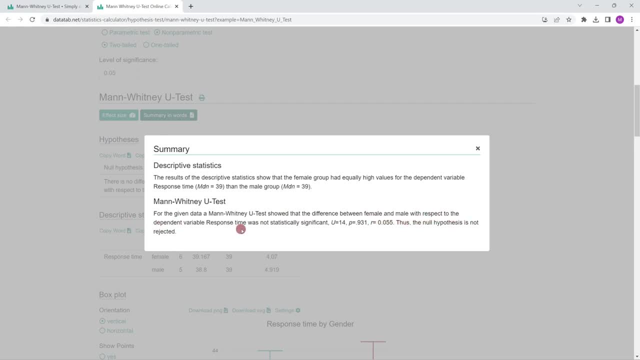 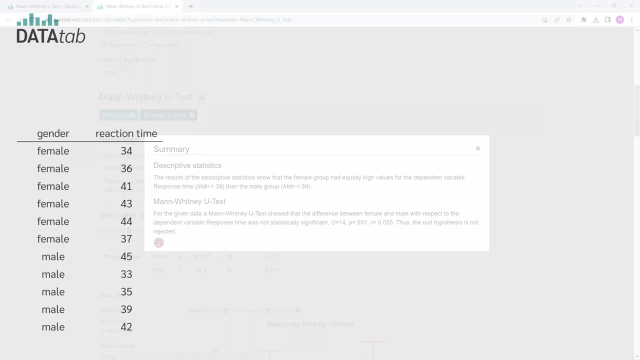 and male. with respect to the dependent variable, response time was not statistically significant. Thus the null hypothesis is not rejected. So we now calculate the Mann-Whitney U-Test by hand. For this we have plotted the values in a table. 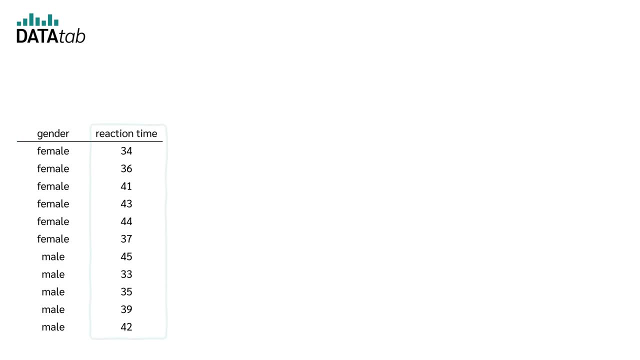 On one side we have gender, with female and male, and on the other side the values for reaction time. Unfortunately, the data is not normally distributed, so we cannot use a t-test and we calculate the Mann-Whitney U-Test instead. 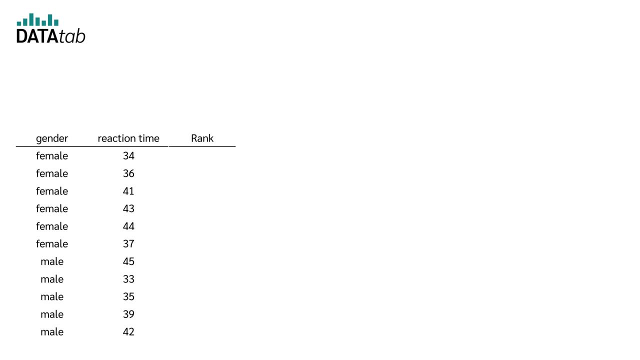 First, we assign a rank to each value. We pick the smallest value, which is 33,, which gets the rank 1.. The second smallest value is 34,, which gets rank 2.. The third smallest value is 35,, which gets rank 3.. Now we do the same for all other. 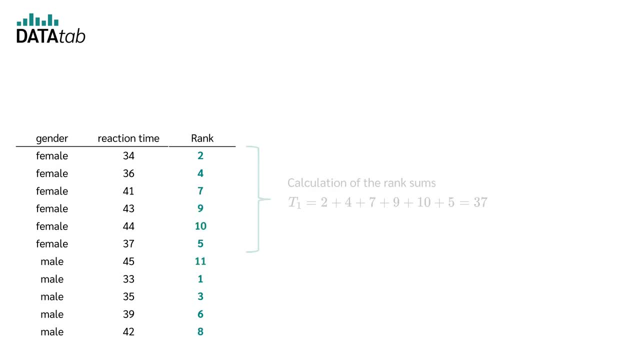 values. So now we have all ranks assigned and we can just add up all the ranks from women and all the ranks from men. The rank sum is abbreviated with t and we get t1 for female with 2 plus 4 plus 7 plus. 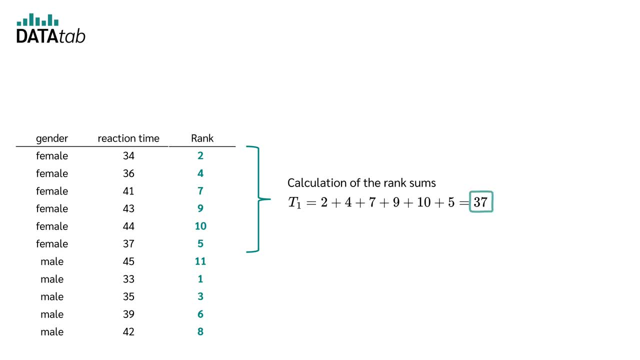 9 plus 10 plus 5,, which is 31.. Now we do the same for male. here we get 11 plus 1 plus 3 plus 6 plus 8, which is 29.. Again, our null hypothesis is that both rank sums are equal. 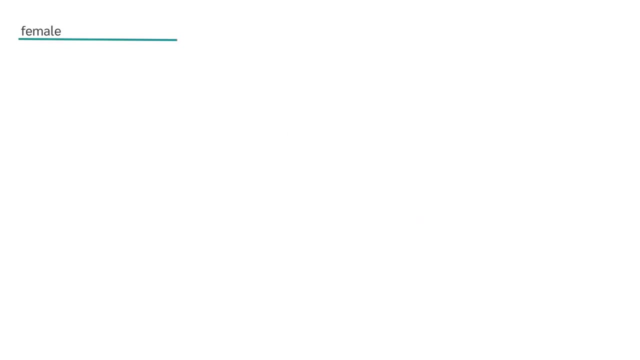 Now we want to calculate the p-value for this. We have once calculated the rank sum for the female participants and we have the number of cases of 6, therefore we have 6 female subjects. We can now calculate the u1, that is, the u for the female participants, using this formula. 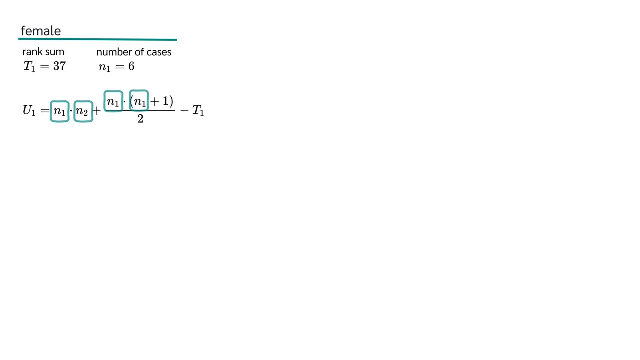 Here we have n1 and n2, that is the number of cases of female and male minus the rank sum of the female participants. If we insert our values, we get a u1 of 14.. We now do exactly the same for the male participants and we get a u2 of 16.. 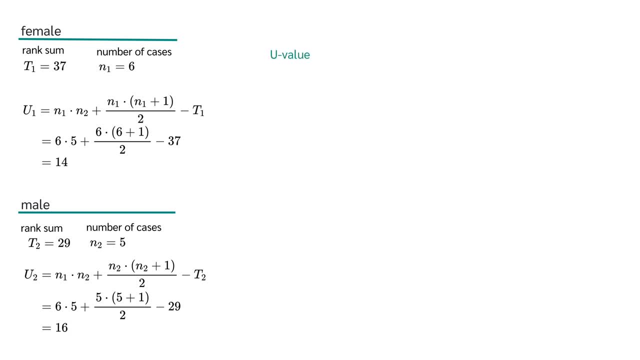 So now we have calculated u1 and u2.. The u for the man with the u-test is now given by the smaller value of the 2.. So in our case we take the minimum of 14 and 16,. this is of course 14.. 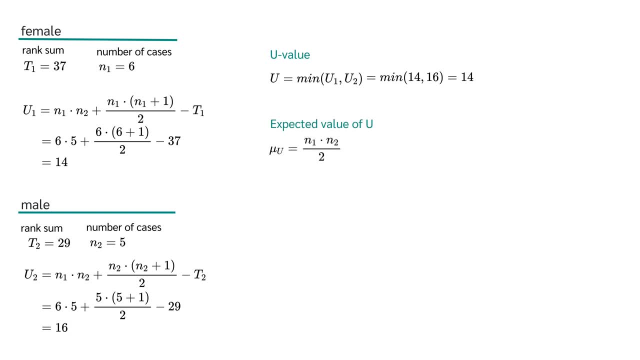 Next we need to calculate the expected value of u, Which we get by n1,2.. Next we need to calculate the expected value of u, which we get by n1,2.. In our case, it is 6 times 5 divided by 2, and that is equal to 15.. 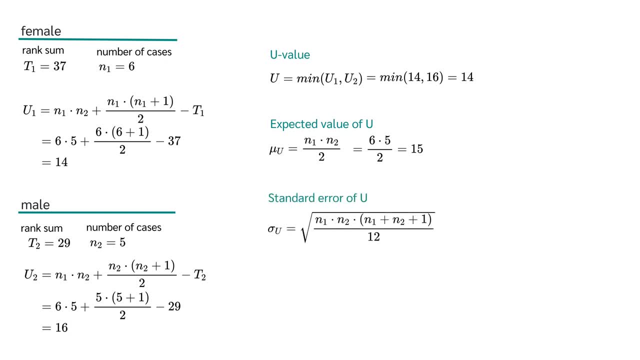 Last but not least, we need the standard error of u. The standard error can be calculated with this formula, and in our case it is equal to 5.4772.. With all these values, we can now calculate z. The z-value results with u-2.. 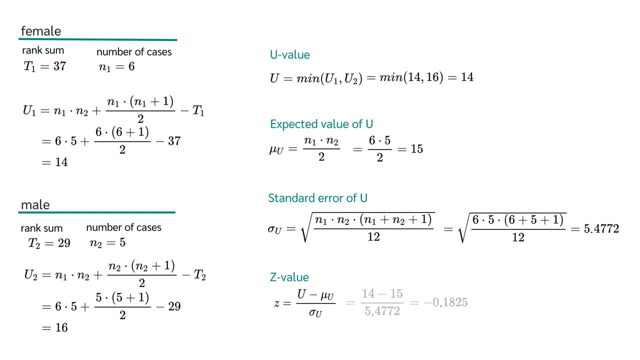 From our case we can get that the z-value is now the momentum p-value. We just need to calculate the z-value. In our case it is 15.. Therefore, equipped with the standard error, we get 16 times 8 minus µu divided by the. 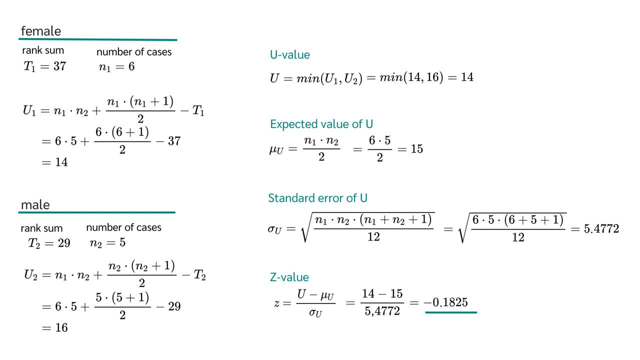 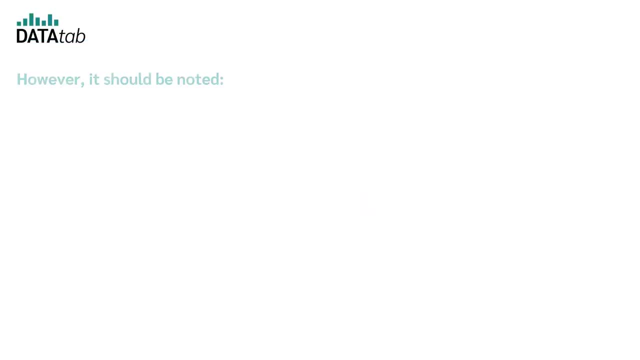 standard error. In our case we get 14 minus 15 divided by 5.4792.. This is equal to minus 0.1825.. So now we have the z-value and with z-value we can calculate the p-value. However, it should be noted, depending on how large the sample is, the p-value for the 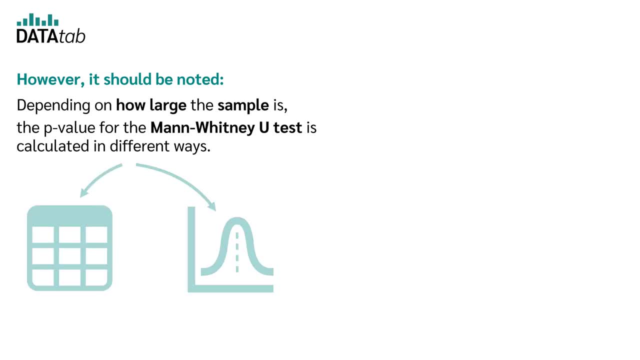 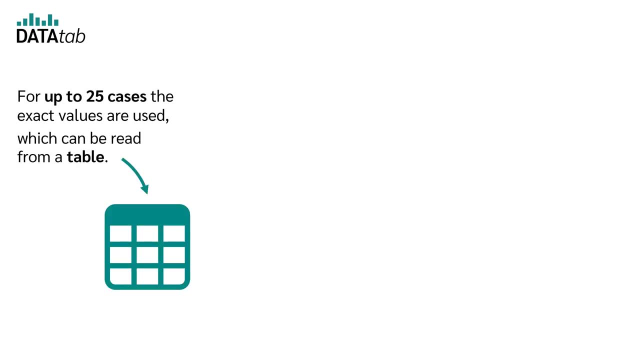 man with the u-test is also negative. So here we did the z-value new test is calculated in different ways For up to 25 cases. the exact values are used, which can be read from a table. For large samples, the normal distribution of the u-value can be used.